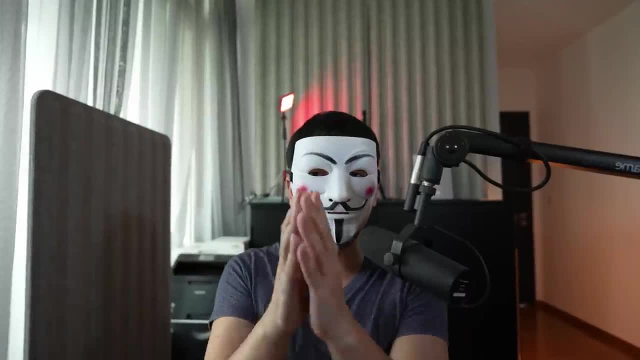 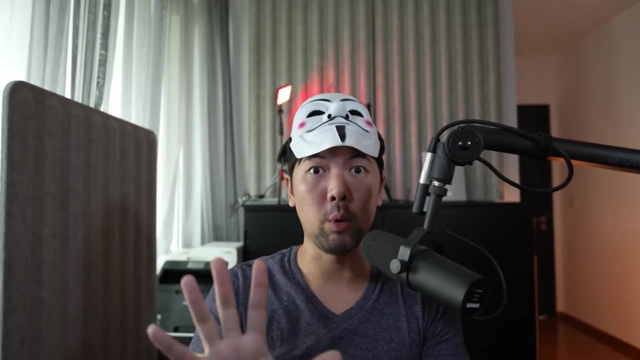 you must hack only the devices that you own. And yes, this video is strictly for educational purposes only. And if I was to send you any files, just go ahead and open it up. I promise you nothing will happen. I mean, just look at, this image is so innocent. What can MrHackAloy do to? 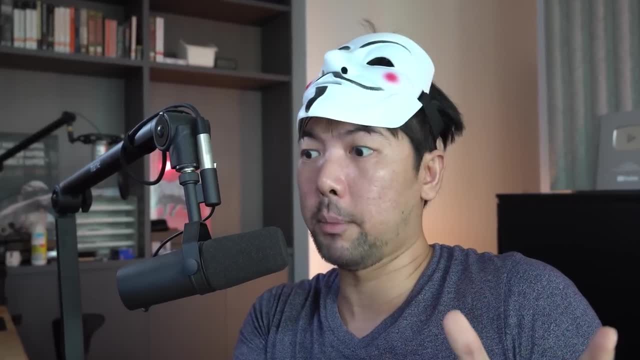 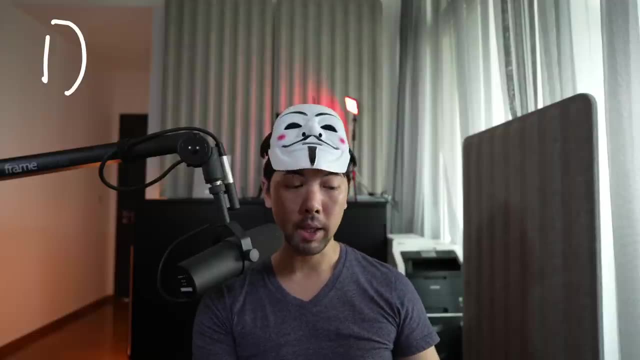 you. I will just help you check what is your email and password and date, above and all the information about you. I'm just doing it for free for you. Okay, just kidding. There will only be three steps for today's session. Step one is you need a photo of someone who is very good looking. 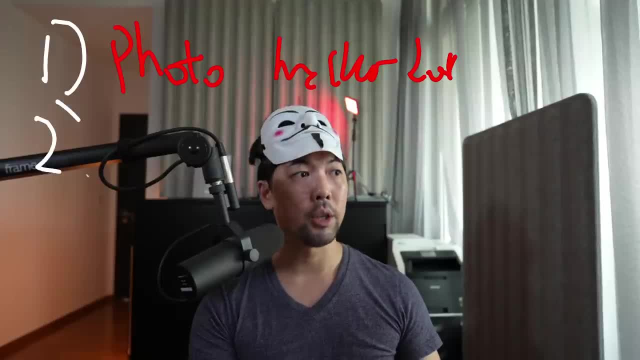 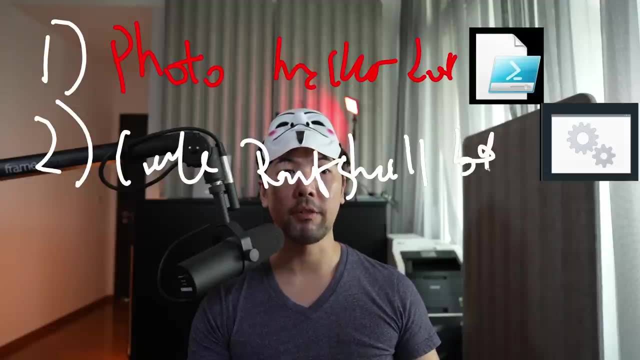 like MrHackAloy. Step two is you need to now write code which is going to be written in, say, PowerShell script, or, at the same time, you can also write in a batch file script. Step three is where we are now going. 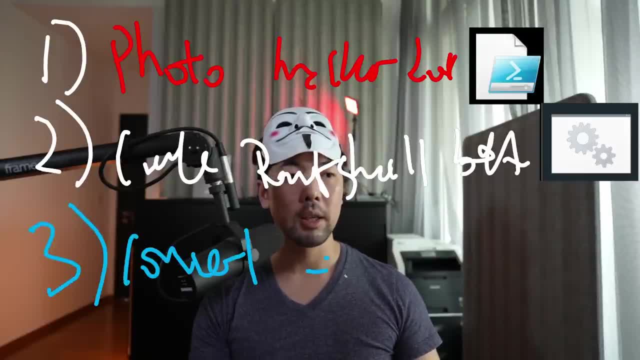 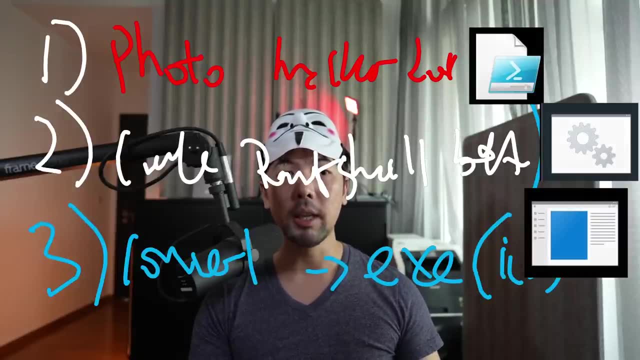 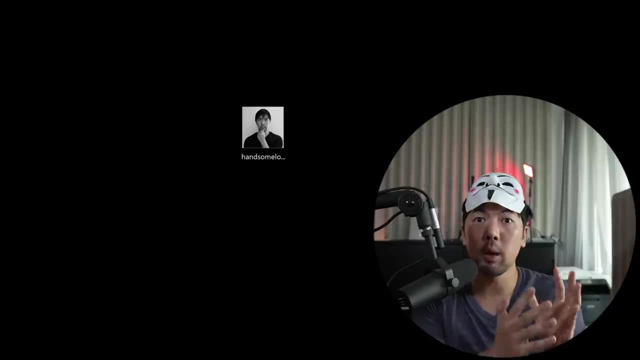 to be able to convert this script that you have written into an exe format that allow us to embed the icon of the image that we've selected earlier into the exe file, disguising it as an image. Well, that sounds pretty straightforward, isn't it? So, as you can see here, I have already downloaded 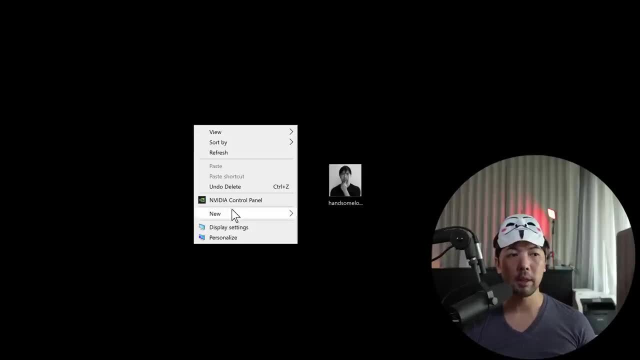 the file. Step three is you need to now write code which is going to be written in, say, PowerShell script or, at the same time, you can also write in a batch file script, disguising it as an image Next up. what we need to do is to go ahead and create a new file. Do a right click. 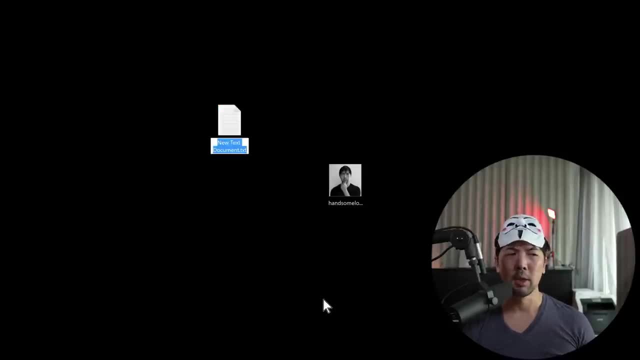 new and go ahead and select under, say, text, dot document. So, whatever the case is, we'll be renaming it. So in this case I'm going to call it as HackerAloyps1,, which is for PowerShell script extension. Hit enter on that And once you hit enter on that, 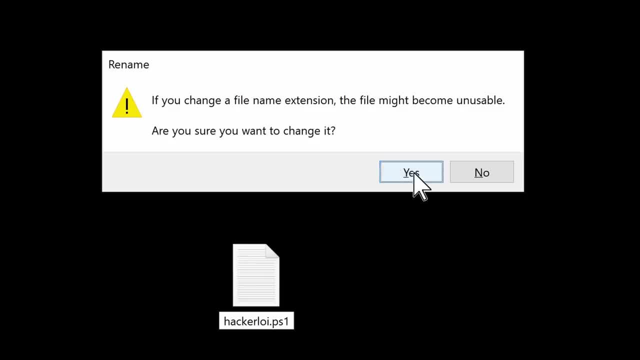 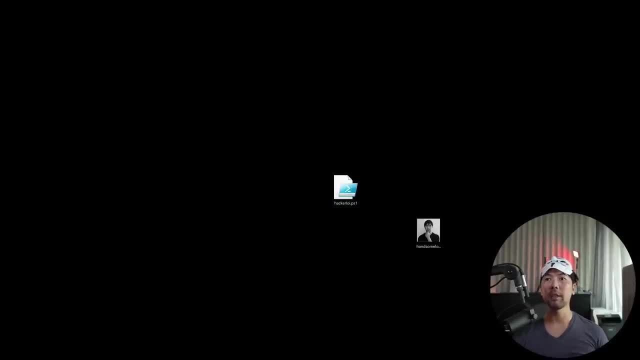 you will get a pop up that says the following: rename: All right, so we're changing the file name extension. click yes, done. And what we'll be doing now is do a right click onto the file, click on add it. All right, so once you click on add it, you can see over here we have oh, oh, oh. 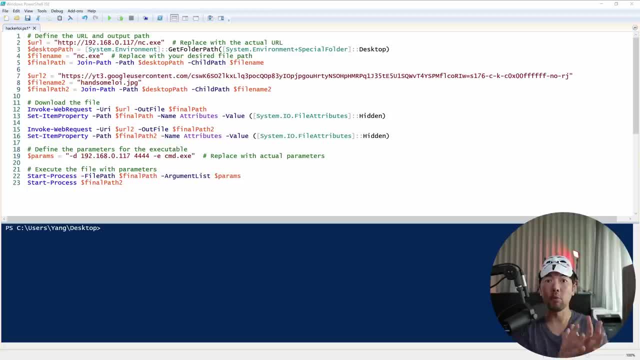 we have Windows PowerShell, ISE. I have already written the code for you and you just have to follow this. it's pretty straightforward. So what we're doing now is we're downloading a specific file called netcat, So this will give us the ability to gain control- remote control- of the. 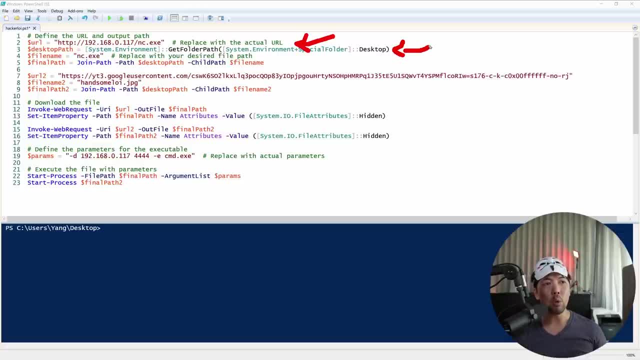 computer And with that, what we're doing here now is to go over into the system environment folder of desktop. So whatever the user is going to be opening file form, we can go into the desktop and be able to launch this application right off of the web. So what we're going to do 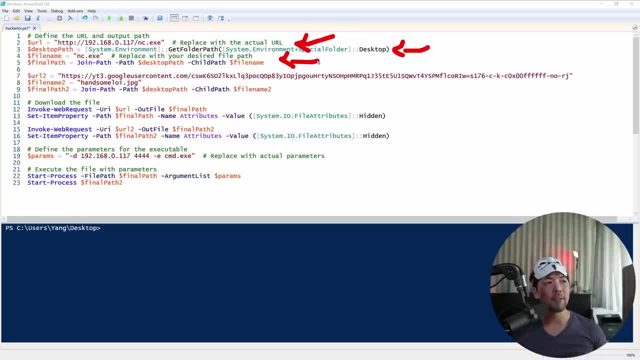 now is open the file and we can go into the desktop and we can go into the application executable. next up we have the file path and, of course, finally, we are joining the file name as well as the path. next up. what we're doing now is to target into the image file of MrHandsomeLoy. 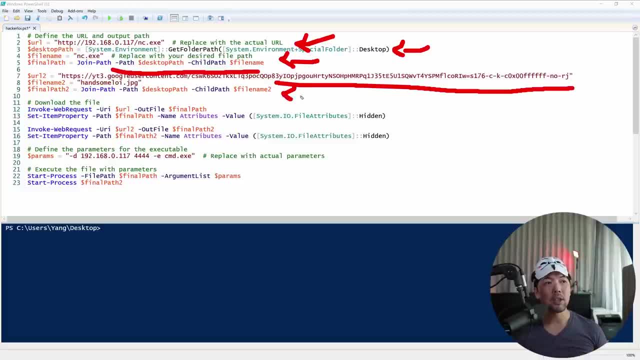 so we're able to download that file and again same thing, save it over into, say, desktop, after which what we're doing here now is we're invoking the uri that we're targeting, all right, and then we're going to hide that file. right same thing for item or object number two, and then after that, 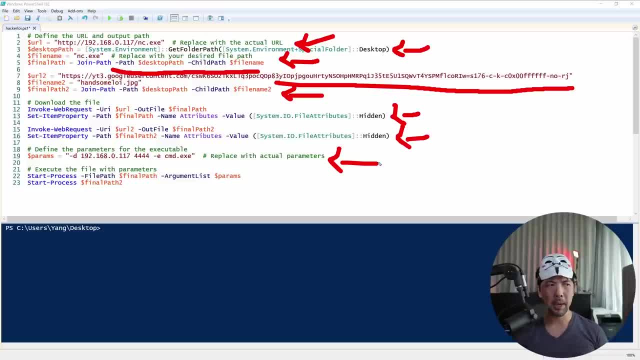 what we do now is we have a special parameter that launches natcat in silent, in the background, connecting over into the hacker's ip address, which then give us that reverse shell and you can see right towards the end. we're executing all of this together along with opening the image. 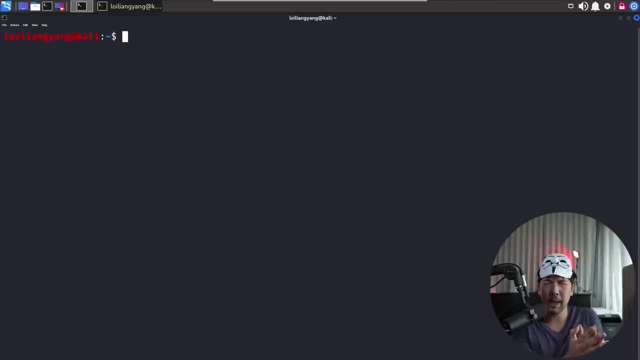 but hiding everything else. and right here we are on our favorite article: hacking operating system, color linux. and all we got to do right now is go and enter, say, nc, nlvp4444, to start our listener so that when the user open up the image, this gives us. 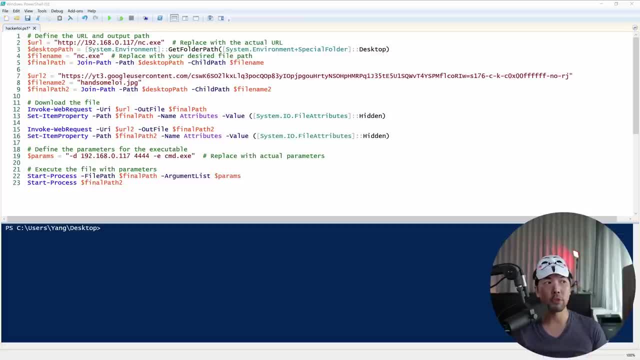 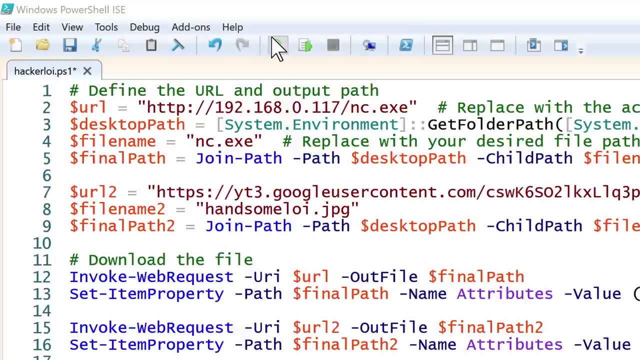 access to the computer. so, going back over in the powershell script, we want to make sure the script is working first before we convert it into an executable. so what we can do now is go ahead and click onto run. the script we are about to run will be saved. click, okay. and then now what we do is we 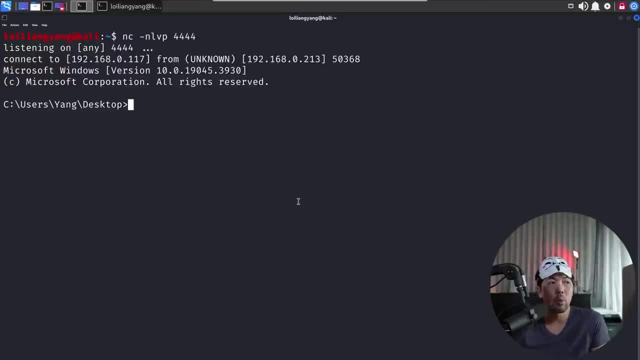 head back over into colin linux and you can see right here we now have access, we now have remote connection to the computer. i can say: enter who are you? all right, just kidding. there's no such command. but i can answer: say who am i? i am pc young, right? so this is hackaloy. and of course at 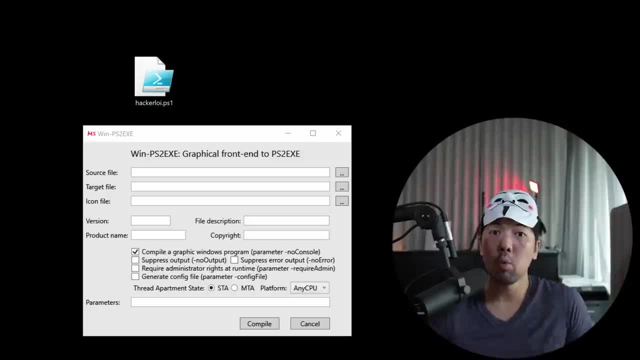 the same time, we have the handsome image popping up right here. so what we need to do now is to convert the powershell script over into an executable. so in this case we have the source file. so let's go ahead and select the source file. so i can do a right click on the source file: click. 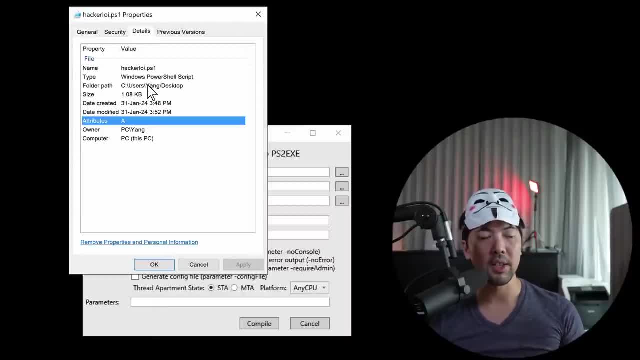 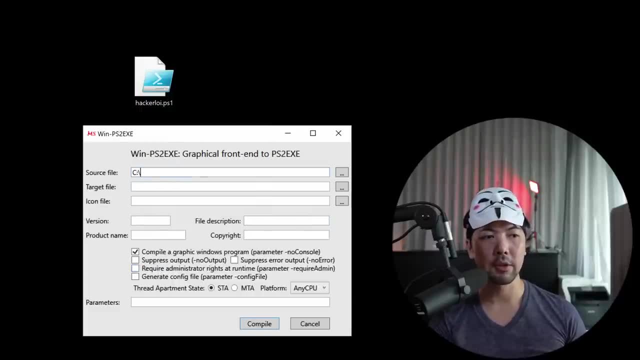 on the properties and over here. all right, we have the details and we can see. that is on see users- young desktop. so go ahead and click on okay. and now what we can do is go ahead and enter the following: our source file: slash- see users- young desktop. slash- hackerloyps1. all right, so target file is going to be c: slash. 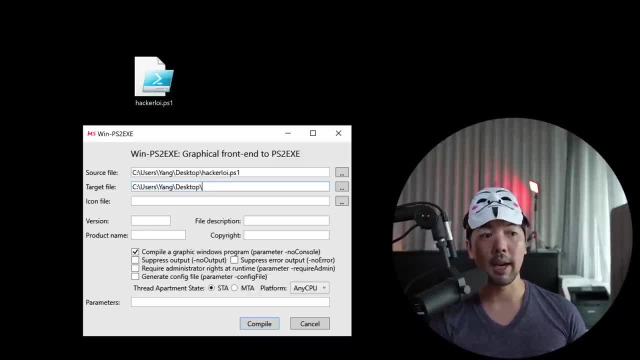 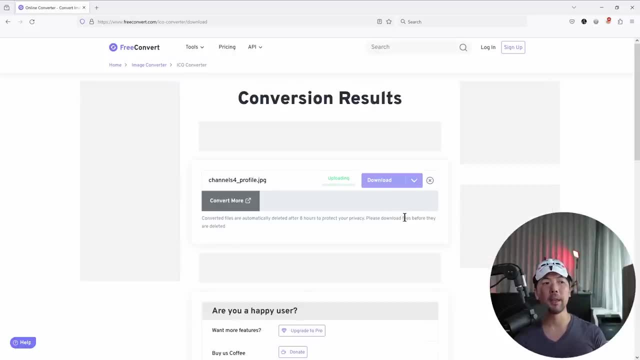 users right, young slash, desktop slash. and, of course, we have the icon file. so what i have here now is the file, and all we got to do is go ahead and click convert into the ico format and we'll be able to download the file. so let's go ahead and download that into our desktop so that we can use. 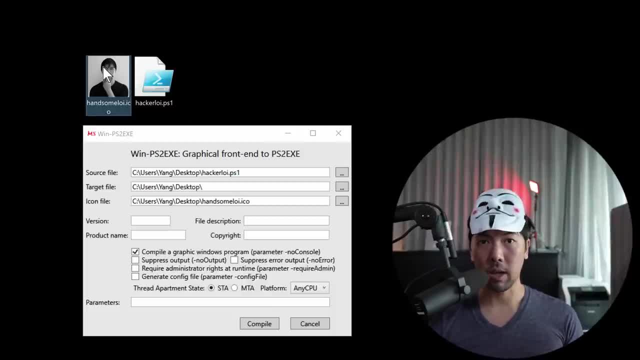 it as an icon. so you can see, here we have the dot ico file and of course we now have highlighted the file, all right, and we have the version, product name and so on, so forth. suppress output. suppress error output. so once you're ready, go ahead and click compile and you can see right. 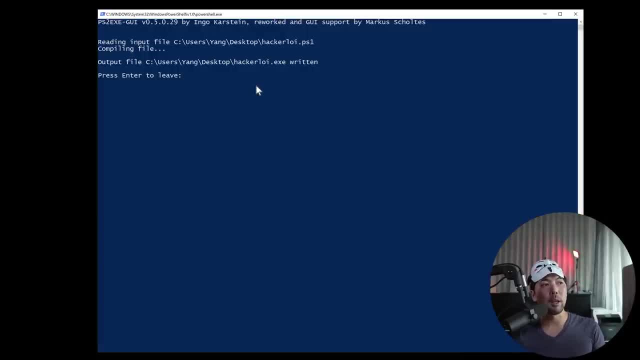 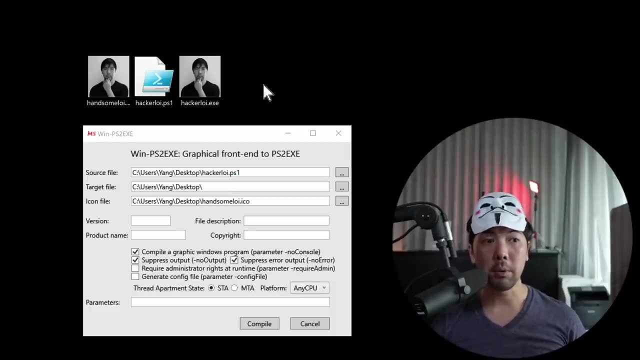 here a pop-up. all right. the pop-up says the following: okay, we're compiling the file and the output file has now been written. all right, go ahead and press enter to leave done. we now have the file. so you can see right here the file has been created. so we can send this file over to. 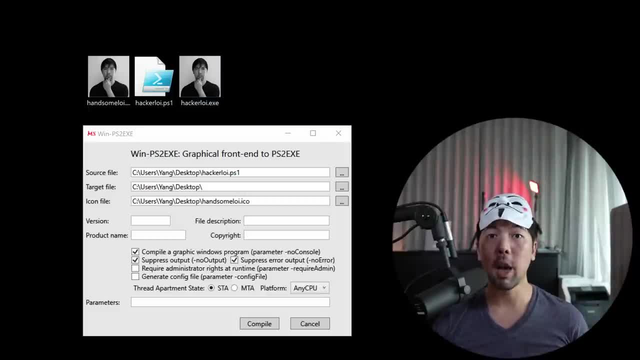 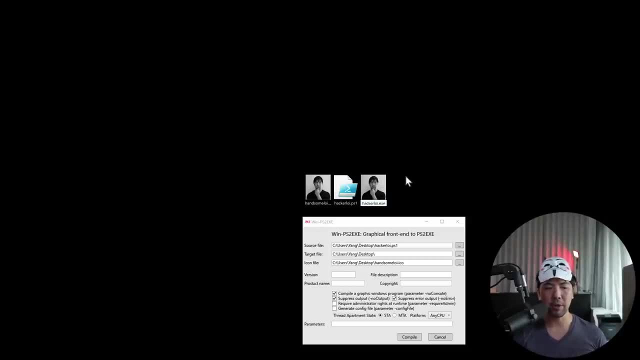 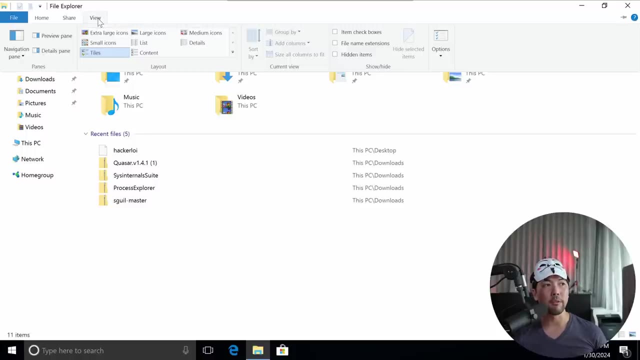 anyone and once they execute under the file, that's it, it's game over. now, before we do that, we need to do right click on this, click rename, and we're going to change the following. so we're going to enter dot, jpg, dot, all right exe. done on most computers if you go on the file Explorer click. 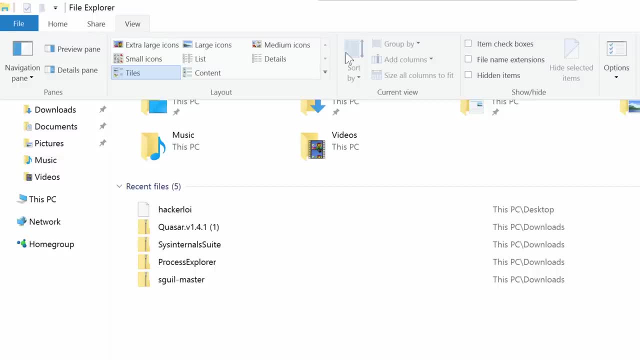 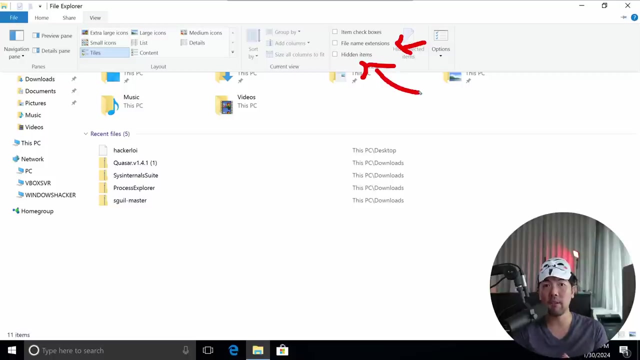 onto view. there are a couple of things that are missing. first is that they do not have the file name extensions being opened up, and number two, they are hiding all these different items. as long as the attribute is hidden, you will be able to hide that file, hide that folder, and this is the. 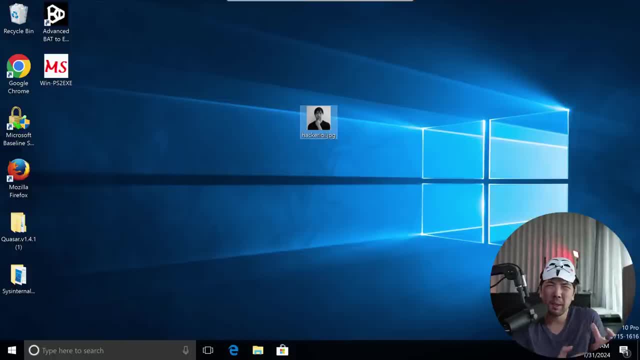 now, as you can see here, we have downloaded the file, and the file can come from an email attachment, it can come from a social media message, it can come from many different places, and what's going to happen now is, if you double clicked on it, it's game over. we'll go back over to colonel Linux and 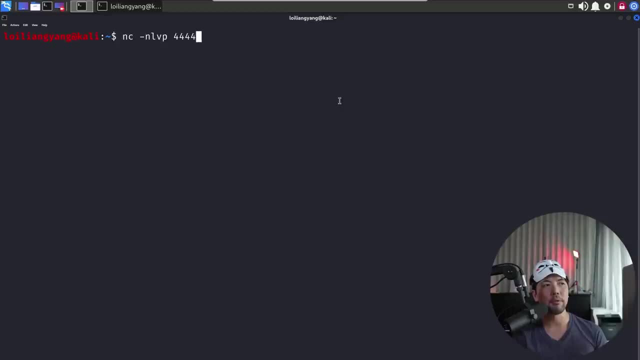 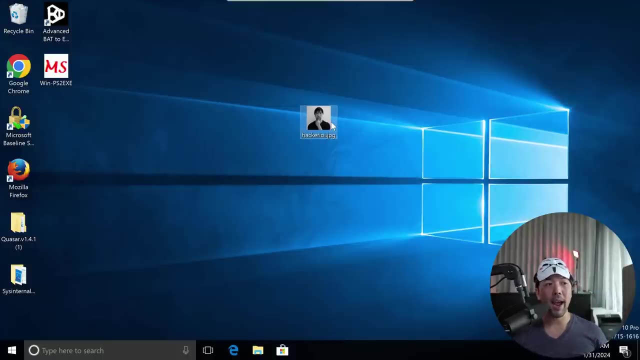 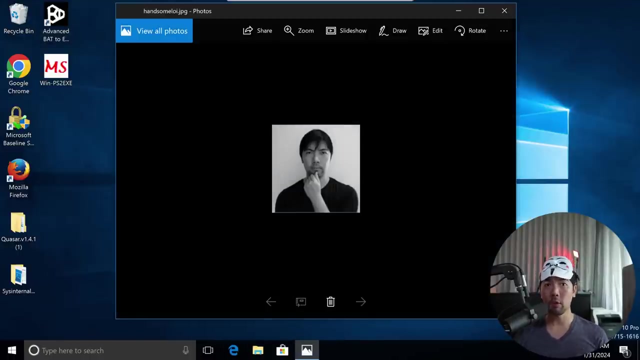 start up our listener. so let's go ahead and enter nc nlvp4444. hit enter on that. so we're listening. our attacker machine is waiting, waiting for connection to come in. now, in three, two, one touch. now. if I go back over to colonel Linux, you can see right here we are in. we now have full.